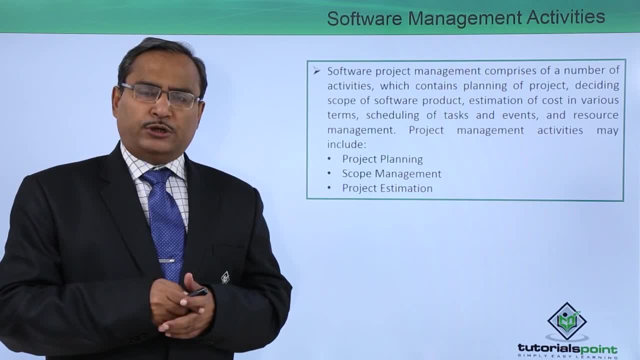 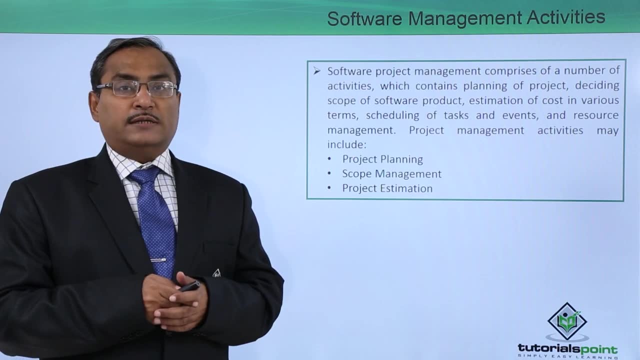 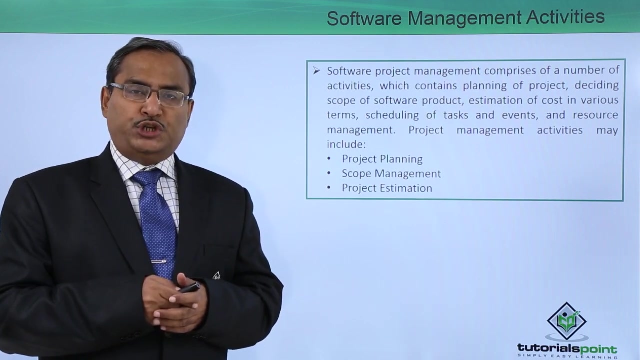 conducted in our project management. we know that a project will be consisting of multiple different phases, as we discussed earlier, and each and every phase will be consisting of certain activities and activities will be comprising of certain tasks. so now all these tasks should be scheduled in a proper way. in between two tasks, there are four different. 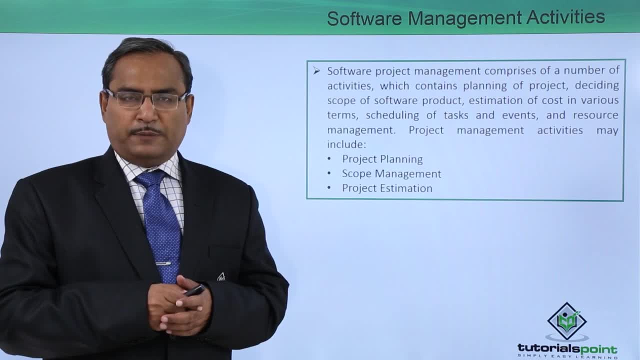 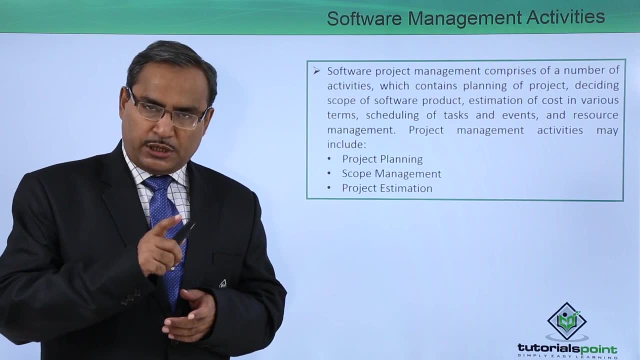 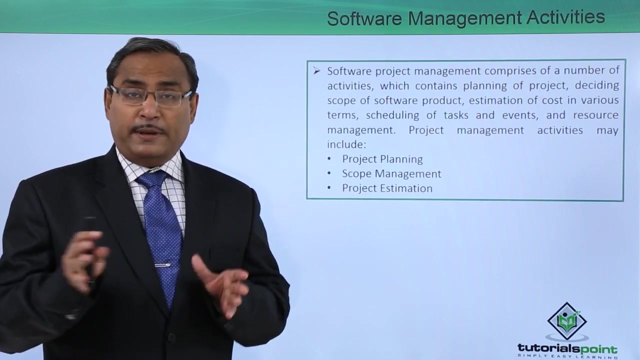 task relationships. that is one is start to finish. that means one task will start after finishing of the second task, then finish to start. one task will finish, then another task will start. start to start. two tasks will start on the same date and time but they may be. 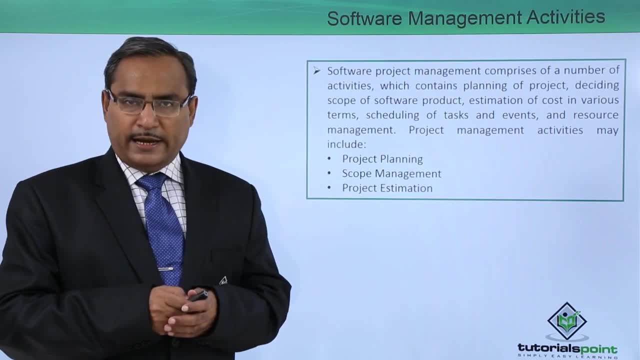 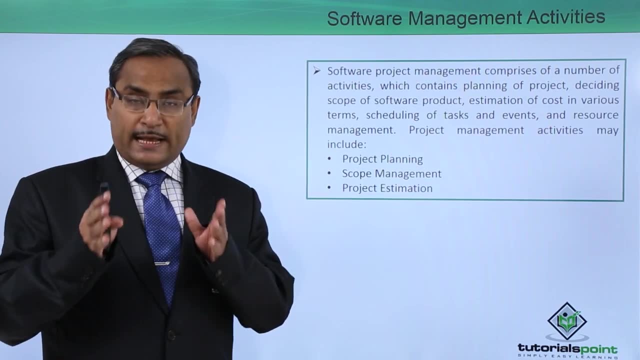 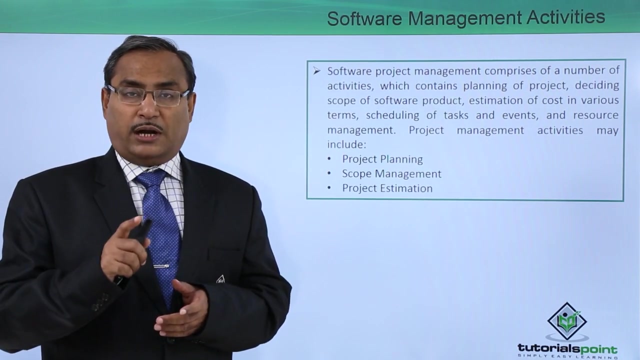 having different durations so they may have different end dates, and another one is the finish to finish. that is, both the two tasks will be finished on the same date and time, but as they might be having different durations, so they can have different start dates. so start to finish, finish to start, start to finish. 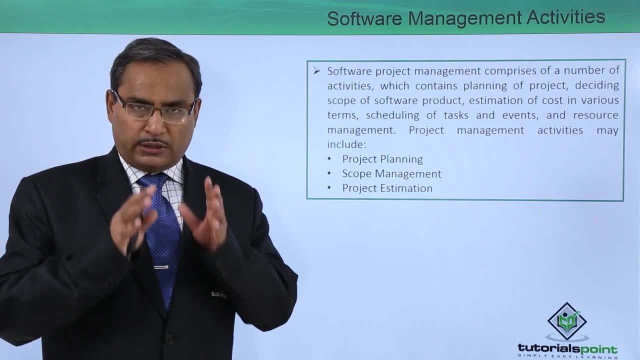 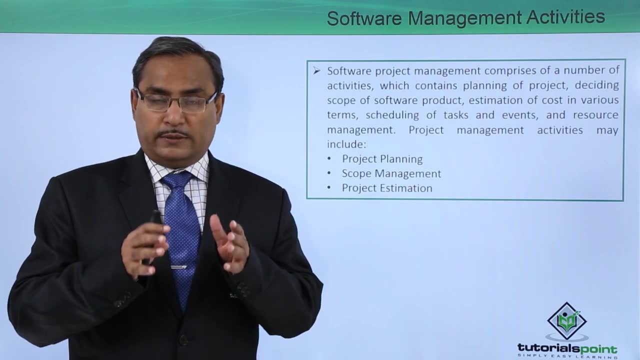 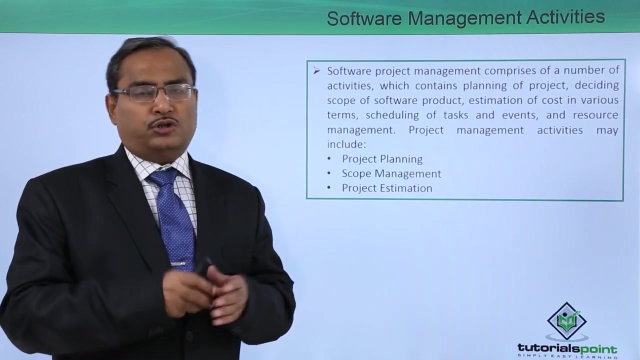 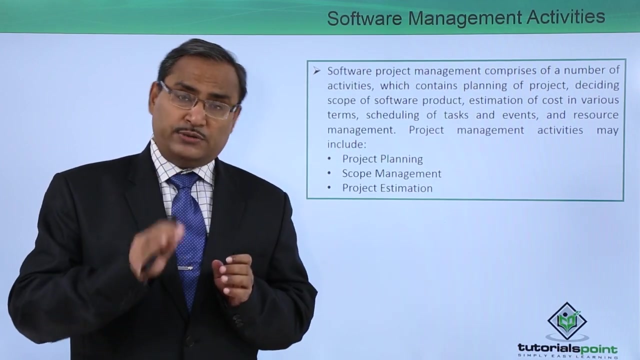 start to start and finish to finish. so there are four task relationships between these tasks and activities. so this task scheduling is a very important, important job in our software project management. and also we shall do the estimation of the cost of the project. we know that tasks will not have any cost. a task will not have any cost. the resources will have. 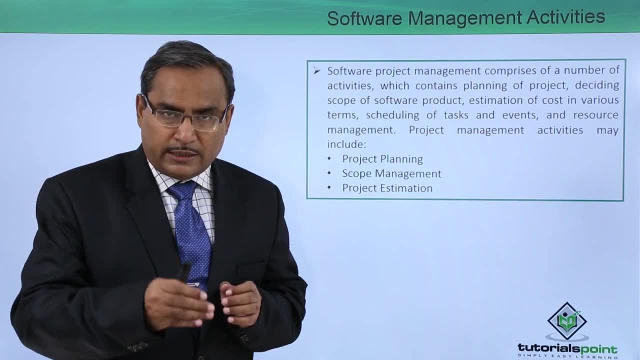 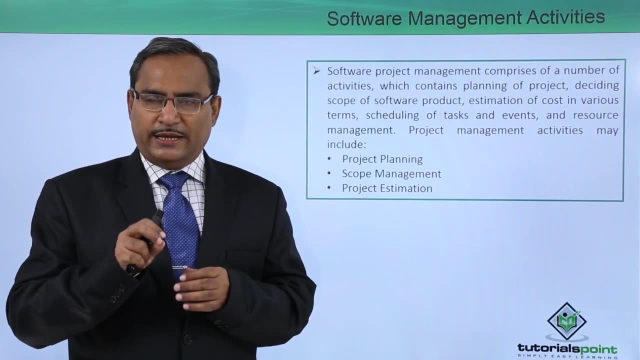 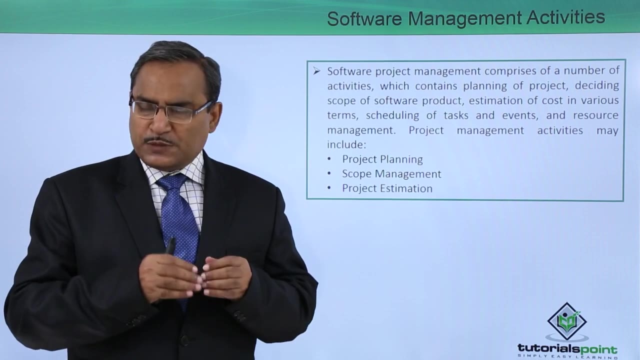 the costs. so when the resources will get assigned on to a certain task, then the task will be have some cost. let us suppose there is a particular developer who is charging x dollar per hour. that is one task which is having a duration of ten hours. so when this particular developer 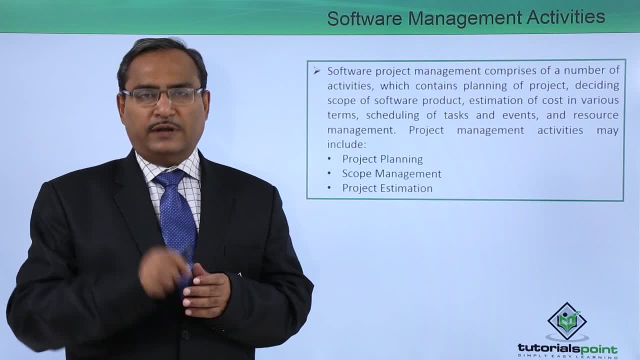 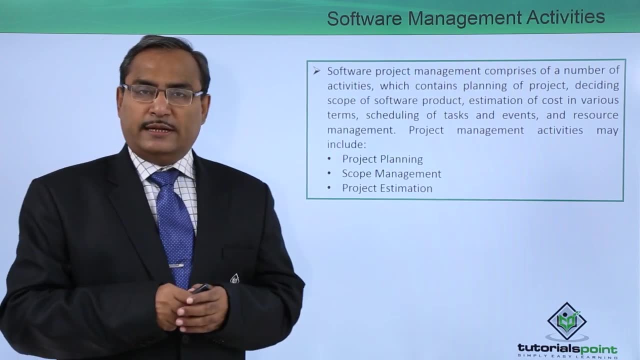 will be assigned to that very task, then the task will have a cost of ten into x dollars. so in this way the task will have the cost. so in case of estimation- there is a estimation of the cost of the project- will be done in this similar way. 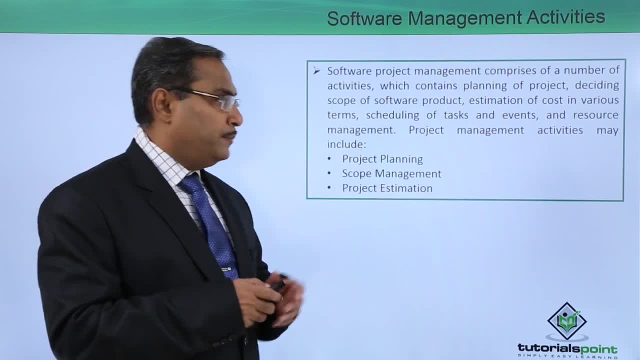 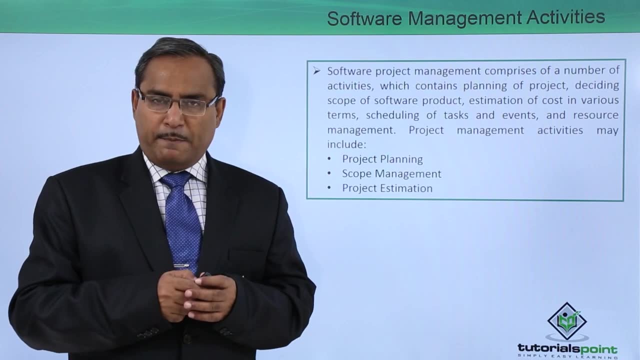 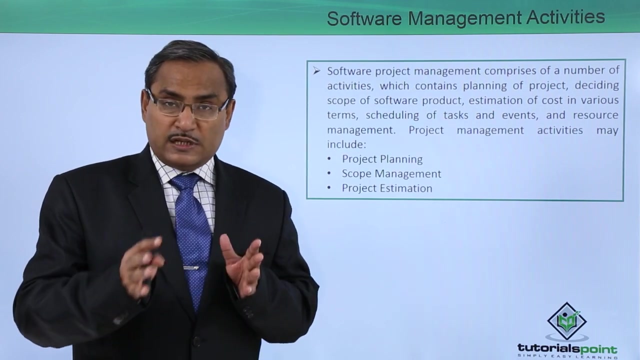 and also we are. we are supposed to do the scheduling of task and events and then resource management. in case of resource management, we are having mainly two issues: one is the over allocation, under, one is the another, one is the under allocation. so what is the difference between? 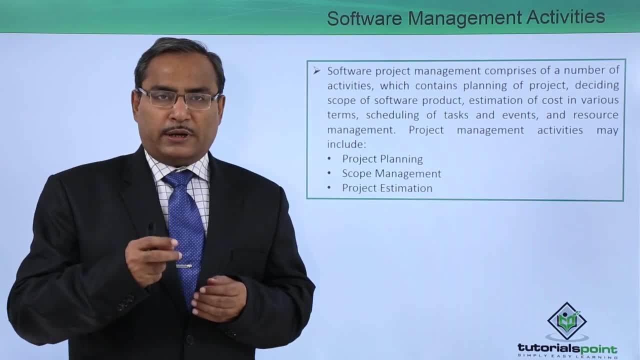 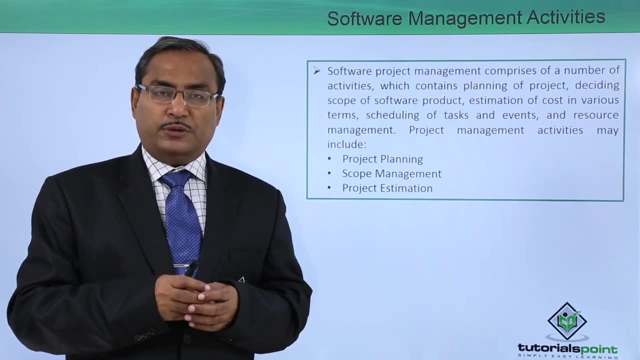 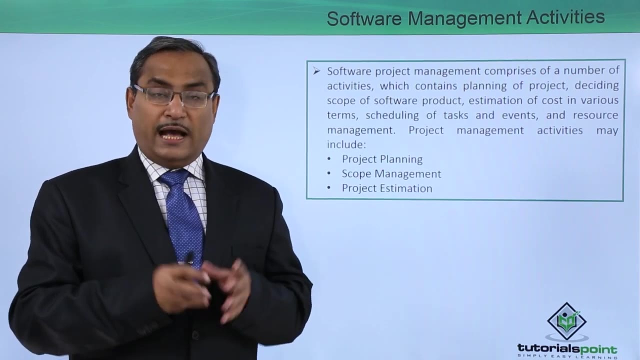 over allocation and under allocation a same manpower cannot be assigned on two tasks on the same date and time, so that is known as the over allocation and under allocation means a resource is sitting idle, but he or she is getting paid, but the resource is not getting utilized, and that is known. 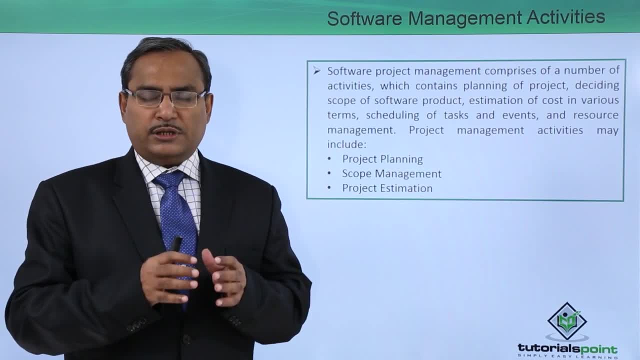 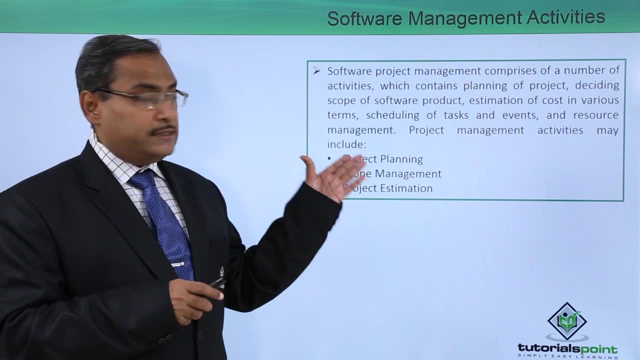 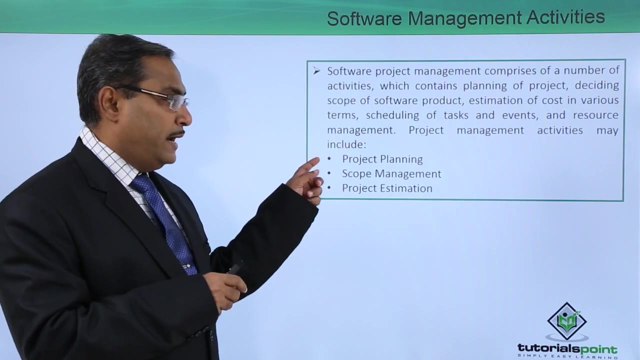 as the under allocation. so all this over allocation, under allocations, all these things are to be resolved in our software project management activities. so, after considering all these things, so let us go forth. so what are the main issues? are there? so project management activities may include project planning, scope management and project estimation. so we are. 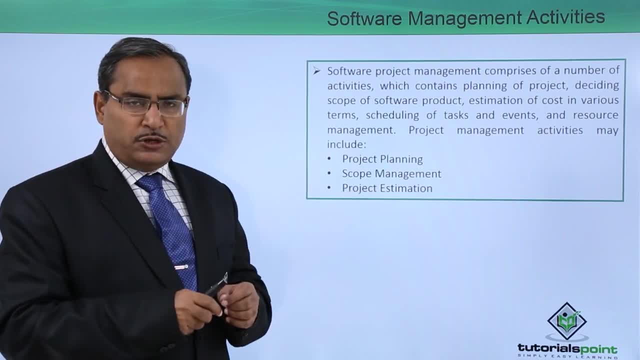 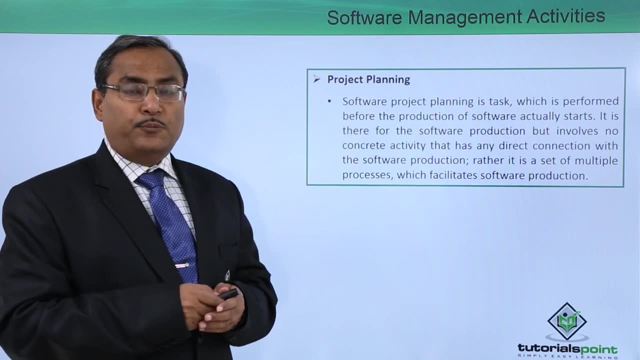 going to have a separate video on project management and scope planning. so we are also going to have a separate video on project management so you can watch that in the future estimation. in this video we are going to discuss on this project planning and scope management. at first we are going to discuss project planning. so software project planning is task, which is. 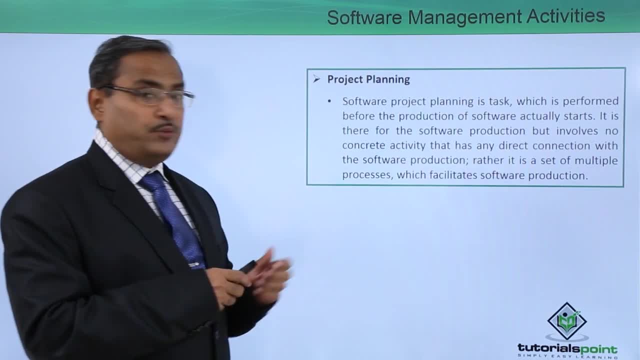 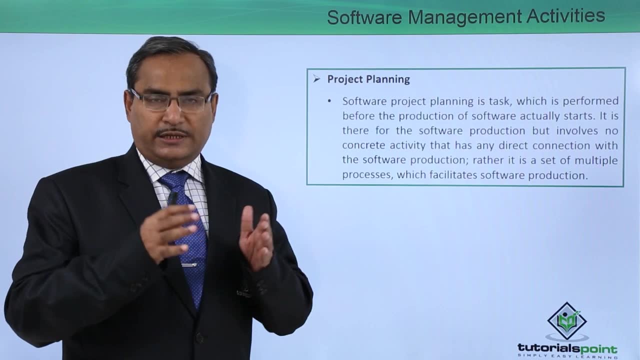 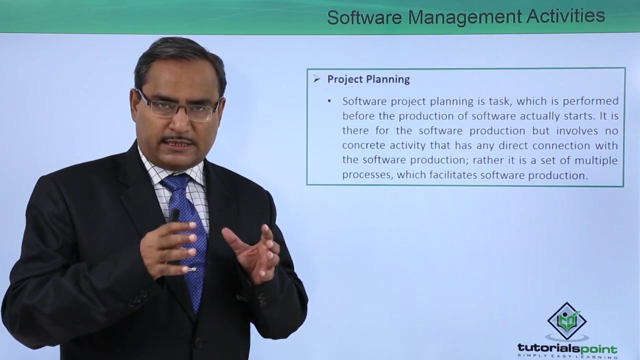 performed before the production of the software actually starts. so that is our project planning. we do the planning before starting the project. we usually estimate the task durations, we try to get what is the nature of the task and we try to do the scheduling of all these tasks and then the 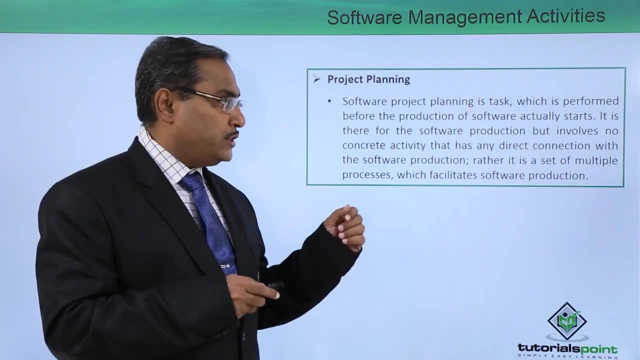 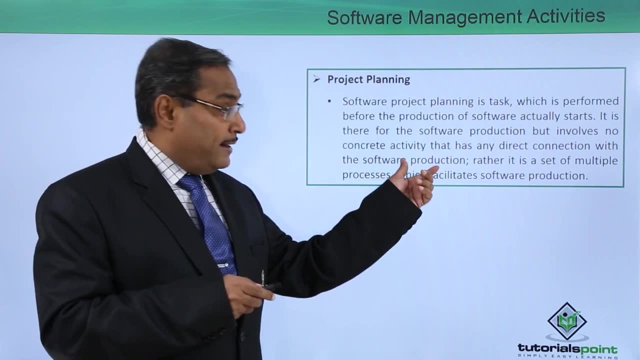 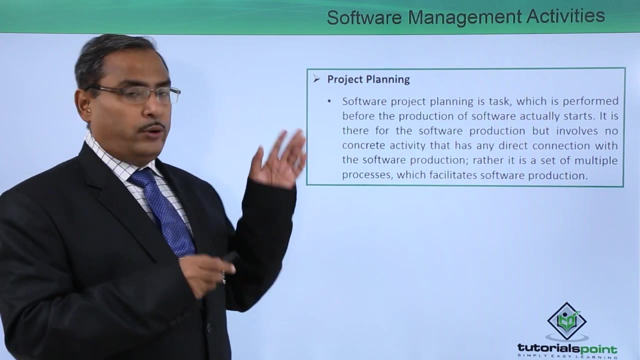 project could get initiated. it is there for the software production but involves no concrete activity that has any direct connection with the software production. rather, it is a set of multiple processes that facilitates the software production. so in this way, we are going to do the project planning whenever we do the project planning, while estimating that task durations. 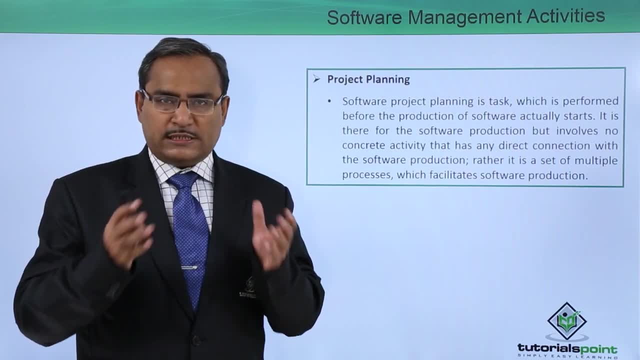 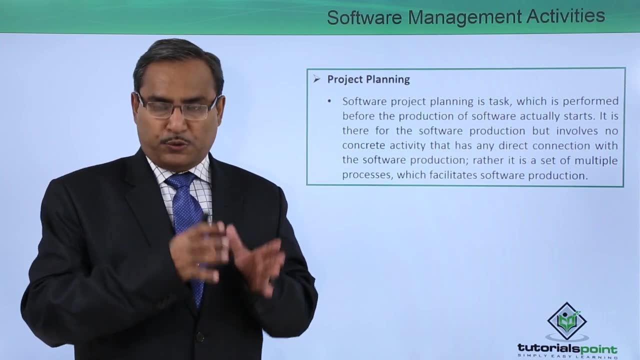 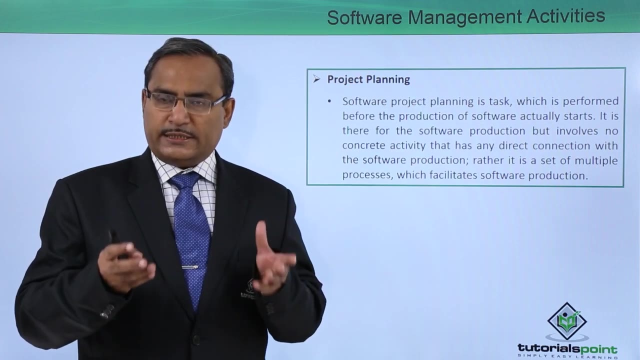 which should remain very much cautious, because we should not over estimate the tax durations. also, you should not do the under estimate. what will happen if we do some wrong during the project planning? when the project will be in execution, the project will be missing the deadlines it will be going to for over budget, under budget, which may also put some 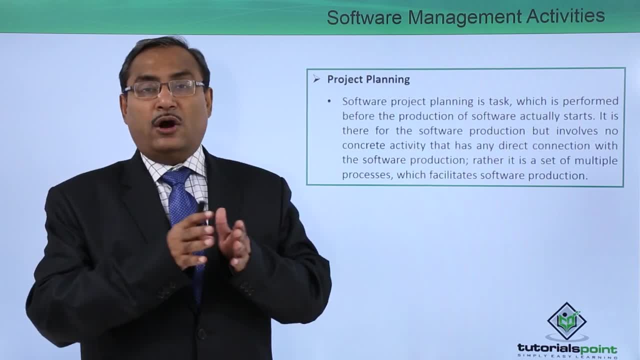 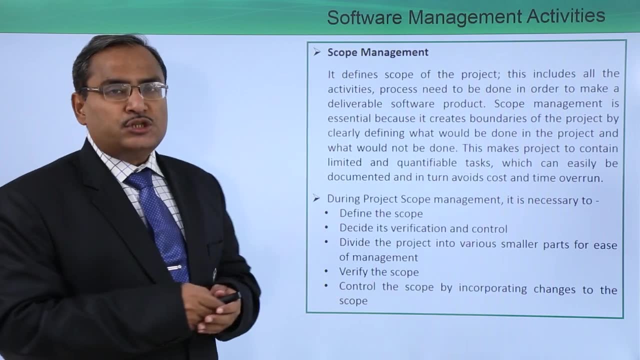 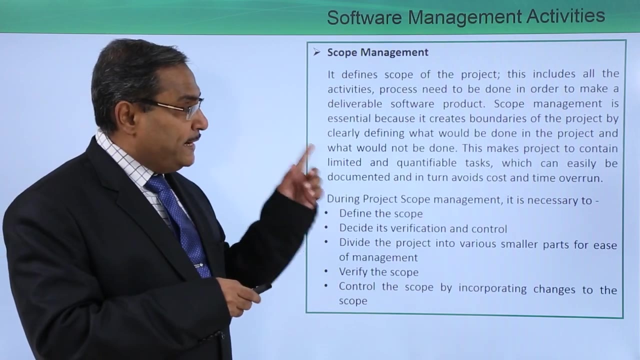 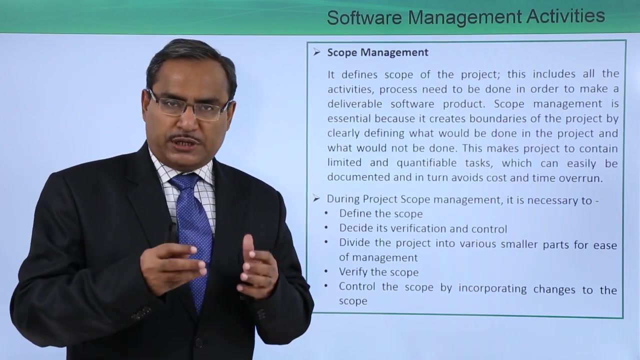 anomalies and some other task are getting delayed due to the elongation of certain task which was estimated with the shorter duration. next one is the scope management, so it defines the scope of the project. that includes all the activities process need to be done in order to make a derivable software product. so scope means different type of features. 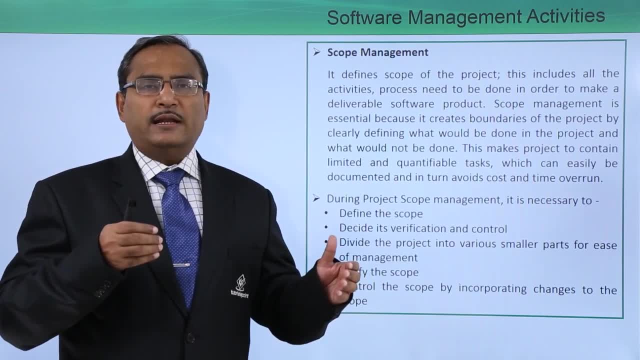 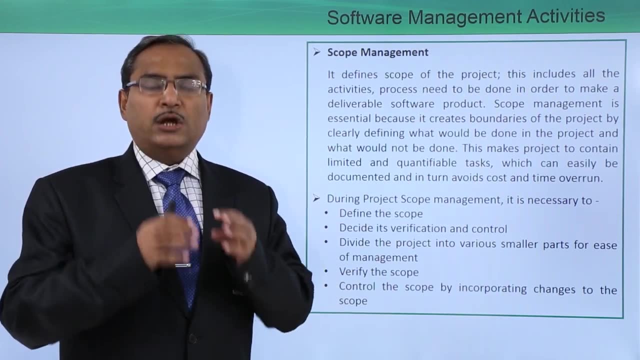 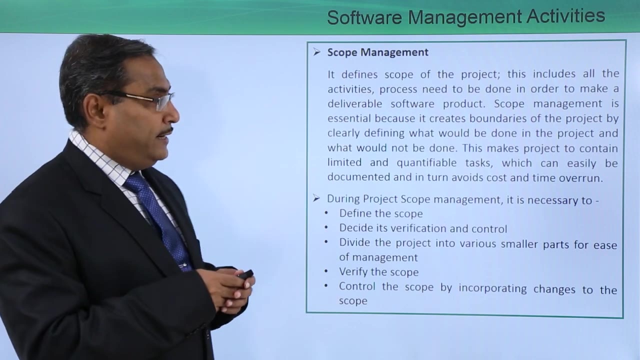 specifications which were decided during the recommend analysis phase, during the analysis phase, software analysis phase, and those recommends. those features are to be implemented during the project, so they will be treated as a scope for the respective software scope. management is essential. it creates boundaries of the project by clearly defining what would be. 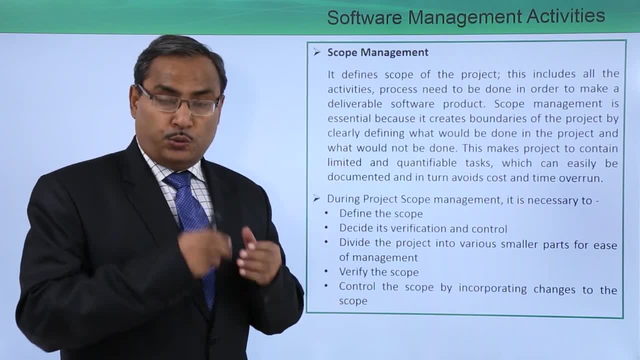 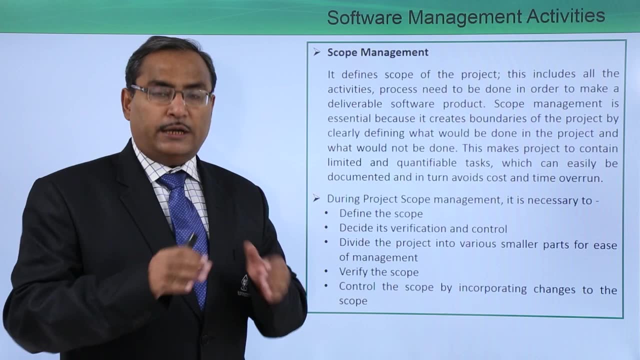 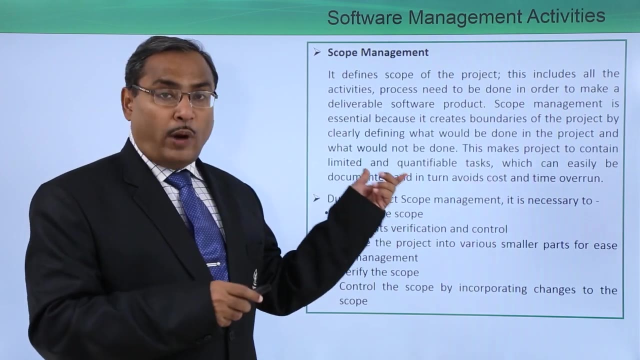 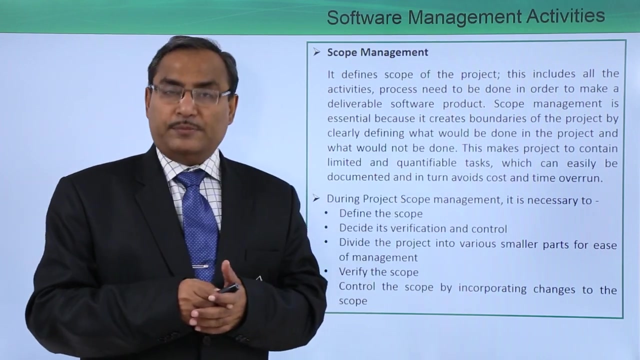 done in the project and what would not be done. so which feature, which scope has to be implemented and which scope should not get implemented would not get implemented, so that boundary will be decided in this scope management, this tax project, to certain limited and quantity quantifiable tasks which can easily be documented and, in turn, avoids cost and time overrun. 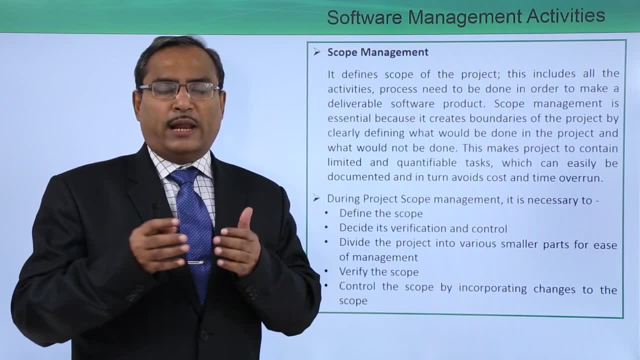 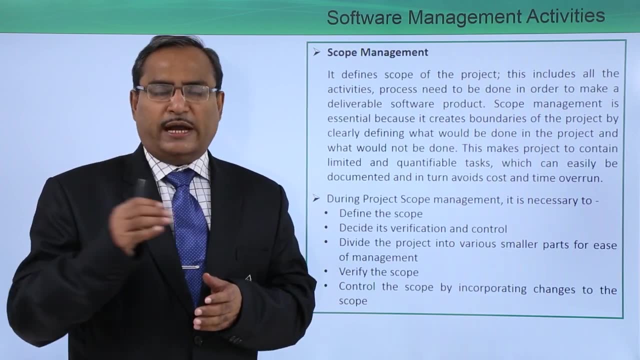 So always we are having a constraint, that is the cost constraint, we are having the constraint called the quality constraint, and another one is the known as the time constraint. So time, cost and quality. So in our earlier video we have discussed this one. that is the 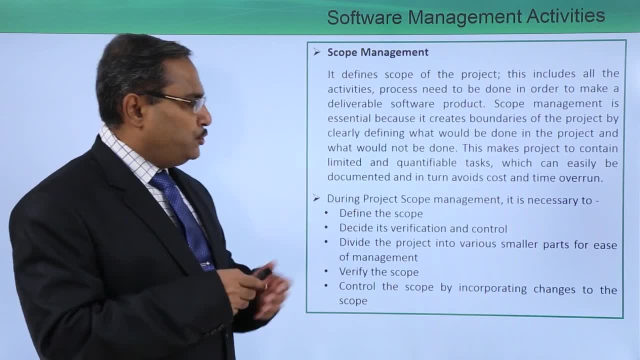 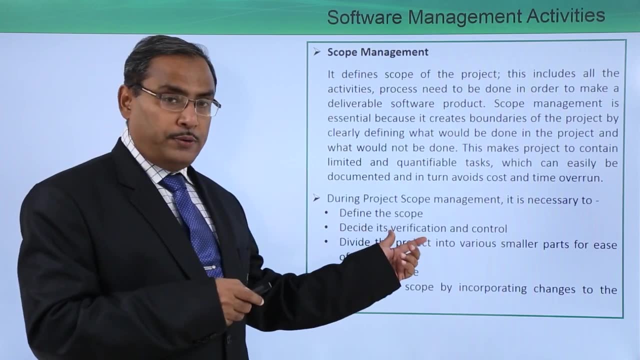 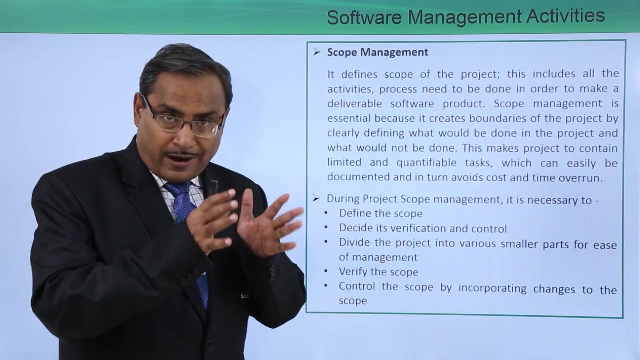 triple constraint in our project management. So during project scope management, it is necessary to. so these are the points I have listed. So define the scope, decide its verification and control, and divide the project into various smaller parts so that it will be easier for. 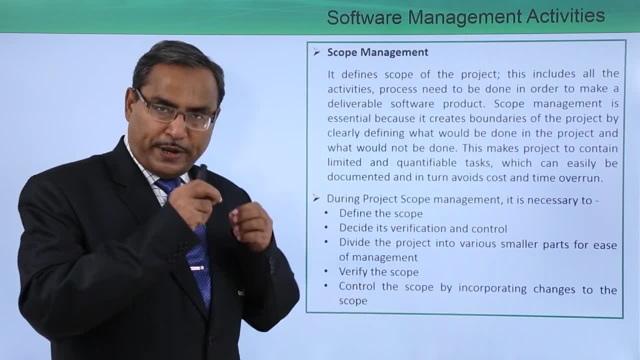 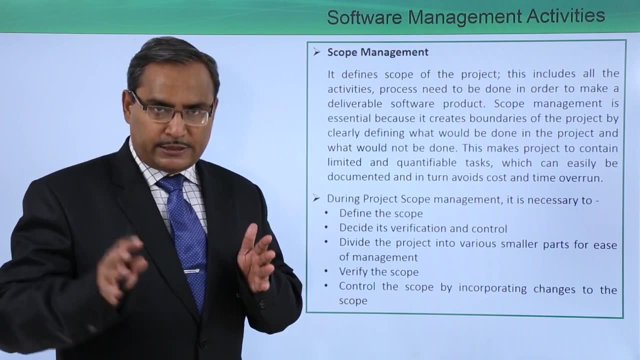 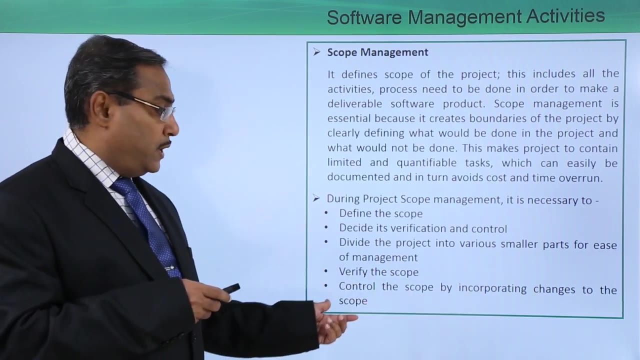 us to do the management and verify the scope. each and every scope is to be verified and it has to be matched with the requirement which we gathered at the early stage of the software development and control the scope by incorporating changes. So in this way we are going to have. this is the list of necessary things to be done. 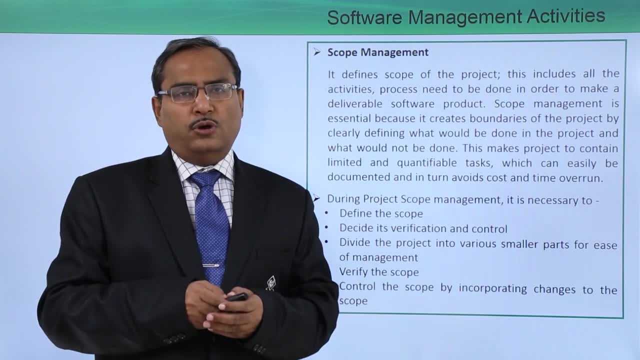 in our scope management. So let us go for the next video, where we will be going for cost estimations. Thanks for watching this.